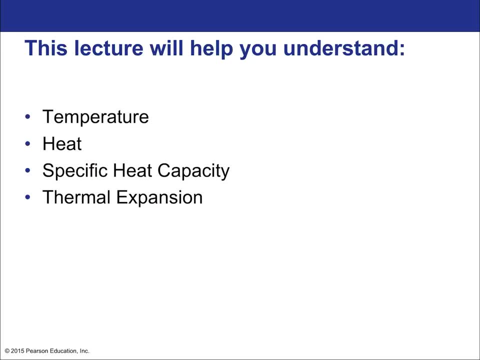 heat and temperature and those kind of related matters. Okay, so just a few topics introduced here. What is temperature? What is heat? All right, how does it differ from something called a specific heat capacity, Because they're really quite different quantities. And then we're going. 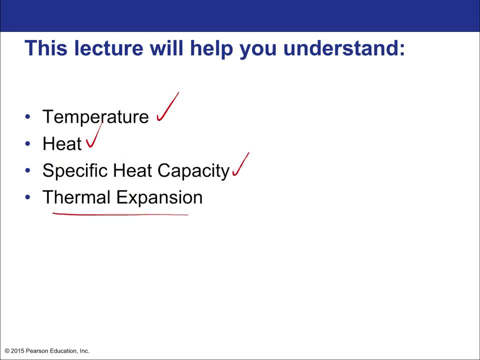 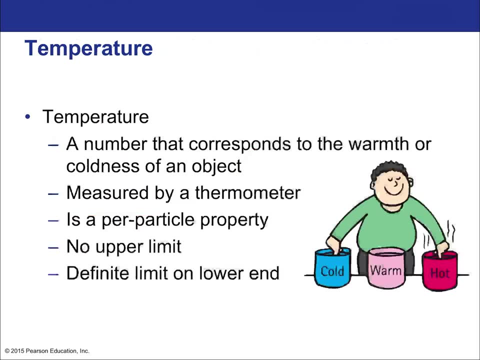 to quantify thermal expansion. so things heating up and getting bigger. Okay, so let's get temperature out of the way. All right. so temperature something we take for granted, but how do we quantify it? It's a number that corresponds to the warmth or coldness of an object. It is measured. 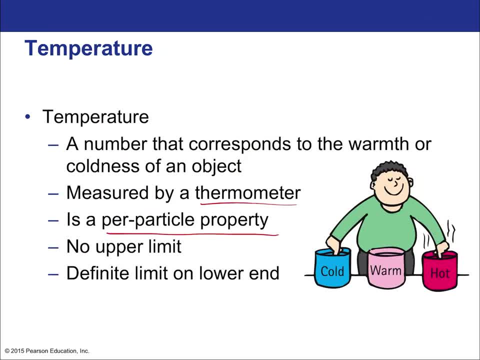 with a thermometer. It is a per particle property. Okay, so it is proportional to the average kinetic energy of the particle. Then make it up So you can think of it as kinetic energy average. All right, it's not equal to the. 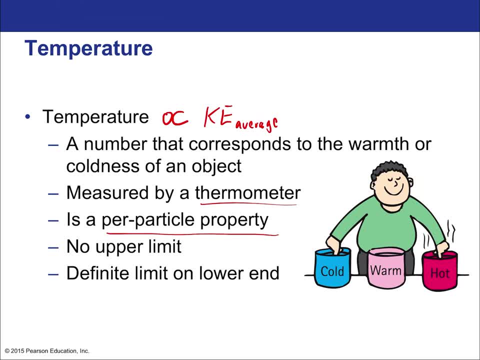 average kinetic energy of the particles that constitute the thing that you're measuring the temperature of, because particles are really small and their kinetic energy is tiny Because, remember, you know, it's one half mv squared but it's proportional to that, Okay, at least to the 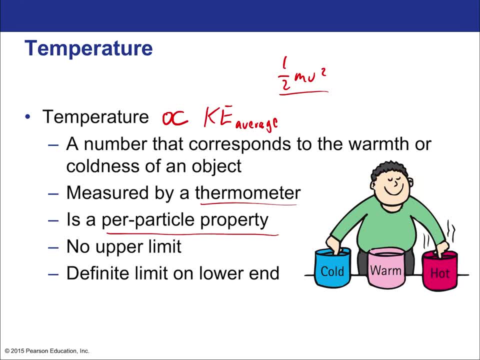 average, And that's really what it represents: some proportionality, Okay, but since it is this kind of unanchored proportionality, it needs its own units. So by introducing the temperature, we're going to introduce a new dimension, a new unit of physics, something we have not done up to. 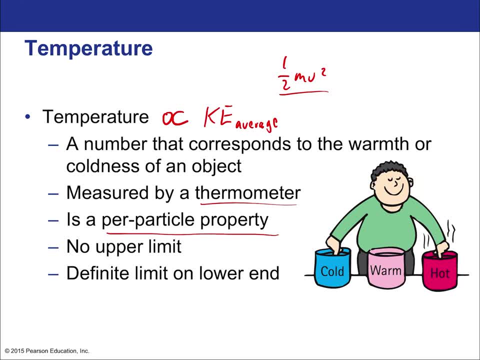 this point. Okay, By the way, there is no upper limit of temperature. My students love to ask me that There are some theoretical ideas about the temperature of the Big Bang being an upper limit, but there's no real kind of agreed upon upper limit of temperature. There is definitely a lower. 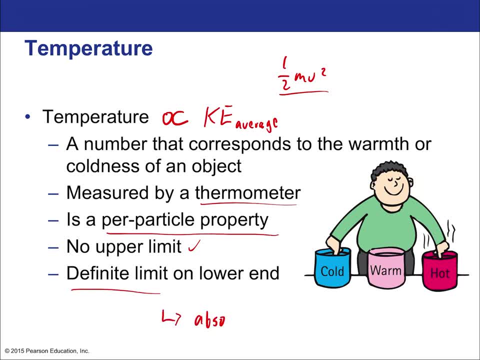 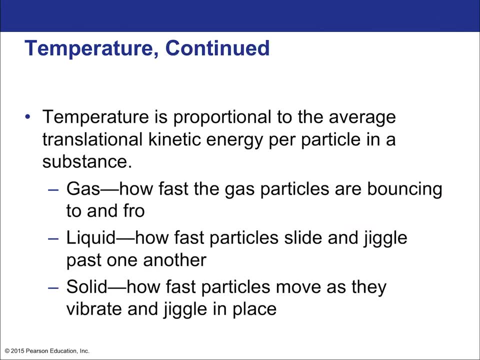 limit. There is something called absolute zero. Okay, we'll talk about that. All right, so let's get into the unit of temperature. All right, So temperature is proportional to the average translational kinetic energy per particle in a substance. Yes, indeed, All right, that's just. 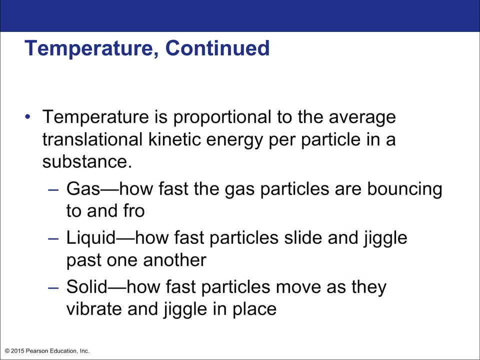 putting into a sentence what I jotted down in the previous slide: A gas. that means that's basically how fast the particles are bouncing to and fro. So that's really, you know, kinetic energy in the sense of a little ball bouncing around. But it also applies to liquids. Those would be the particles. 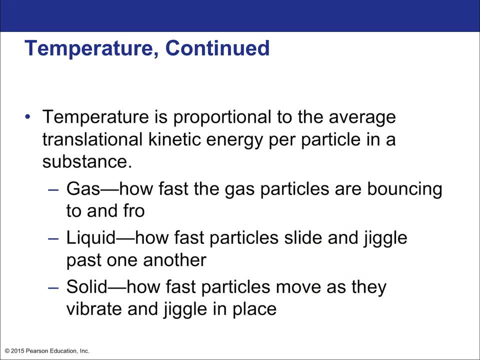 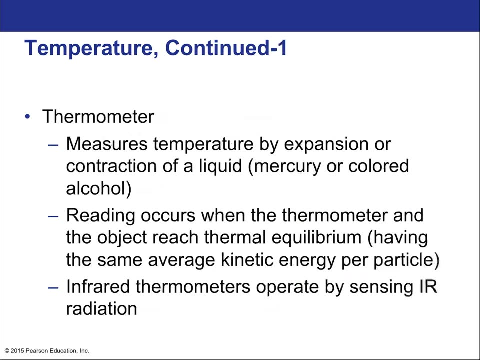 sliding together the sort of the sheets of loosely connected molecules And for a solid you can think of a lattice of molecules all interconnected through their molecular bonds jiggling around. Okay, So again, a thermometer measures temperature by expansion or contraction of a liquid. So it 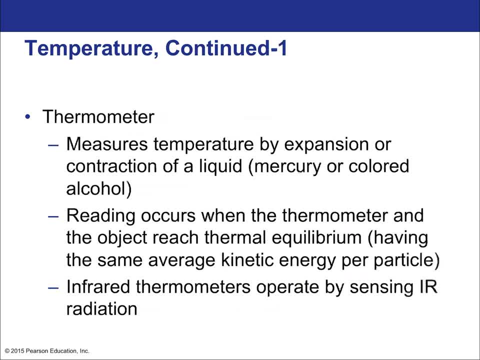 uses the last topic of this chapter, thermal expansion, in some quantifiable way. It's basically calibrated, Okay. So it's calibrated so that those changes mean something. If you think about a digital thermometer, it can use other mechanisms. It can use electromagnetic mechanisms. 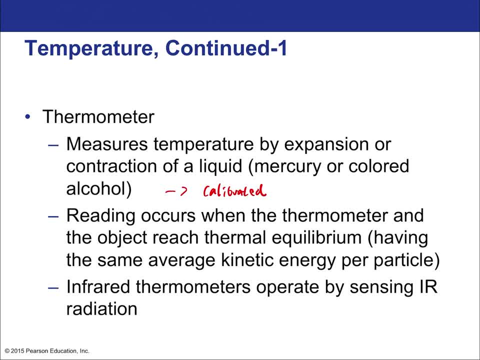 such as a change in resistivity of a wire, a temperature dependent resistivity change. That's actually a very, very common way to measure temperature. That's also a good way to measure wind speed because of its association with wind chill. Furthermore, temperature can be measured through means of other you. 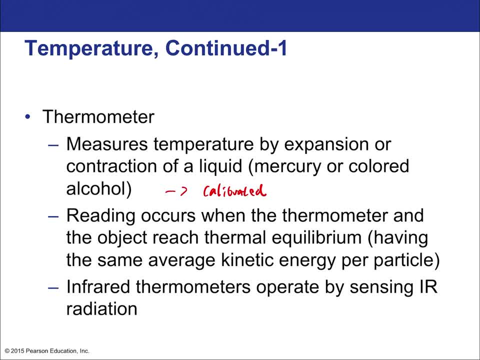 know, like other circuitry elements, But resistivity is by far a really simple way of measuring temperature. Okay, But a more old fashioned and kind of fundamental way would be this idea of thermal expansion. Okay, Reading occurs when the thermometer and the object reach thermal equilibrium. All right, That's when they're both the same. 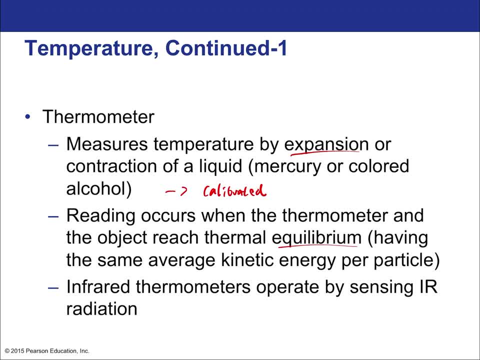 temperature. That's not necessarily instantaneous. Okay, Think about a meat thermometer: It takes a minute for it to reach equilibrium. And infrared thermometers operate on another principle: They operate by sensing a particular radiation. How does that correspond to temperature? Well, we'll talk about that a bit when we talk about properties of light. But the key word 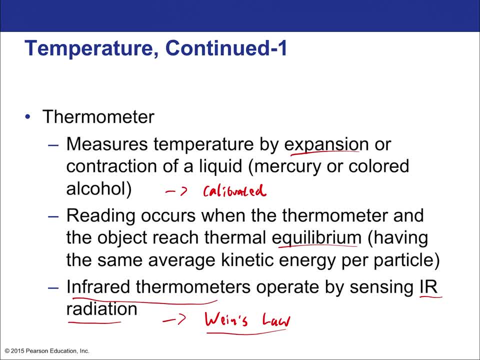 here is something called Wien's law, which is something I always cover in my astronomy classes, But it's a really amazing law And it only applies to solids. It doesn't work for gases, by the way, or liquids, But it tells you that color means. 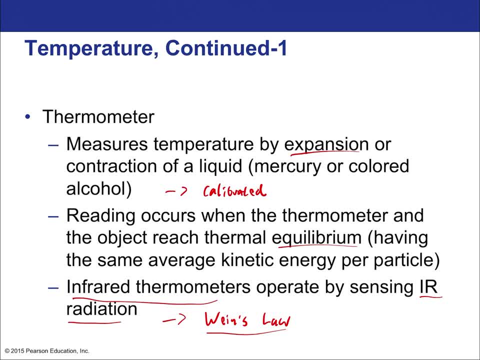 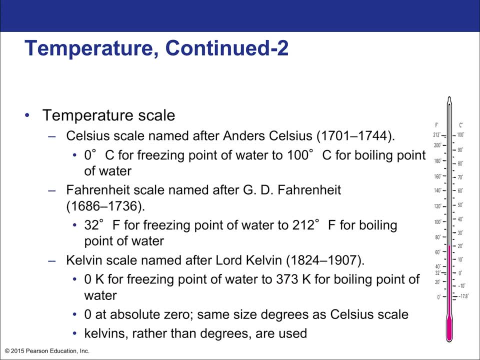 temperature. There's a direct relationship. There's a functional relationship between the two, which is remarkable. It's not perfect, but it is pretty darn pretty good relationship between the two. Okay, All right. So let's get into those temperature scales, right? That new unit? I? 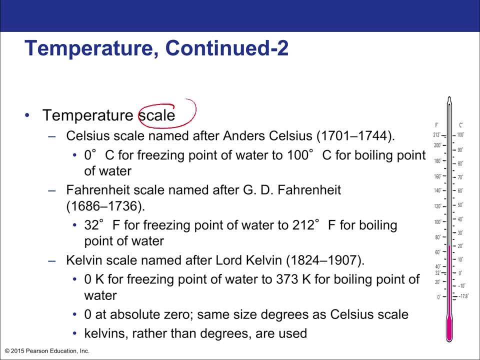 mentioned. Okay, So first of all, let's go. Let's start with the oldest temperature scale first, which is the second one down the Fahrenheit temperature scale. Okay, So this was developed by a man here that lived between 1686 and 1736. And this temperature scale has 32 degrees as freezing and 212 degrees for boiling water, which 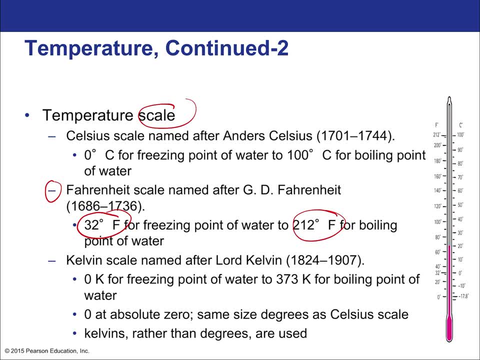 seemed like really weird choices, But that was not the purpose of the Fahrenheit scale. The Fahrenheit scale was meant to be a anthropocentric type of temperature scale, And anthropocentric just means that it's human focused. So, essentially, a change in Fahrenheit is really easy to recognize. The temperatures that we tend to experience- as you know, earth weather- are going to fall in numbers that make intuitive sense to us. I mean, just think, for example, that a one degree change in Fahrenheit is a smaller scale than a one degree change in Celsius, the next temperature scale we're just about to talk about. That means it's more granular And that's better for actually describing the human experience. If I say the difference between 30 degrees Celsius and 31 degrees Celsius, well you know that's a. 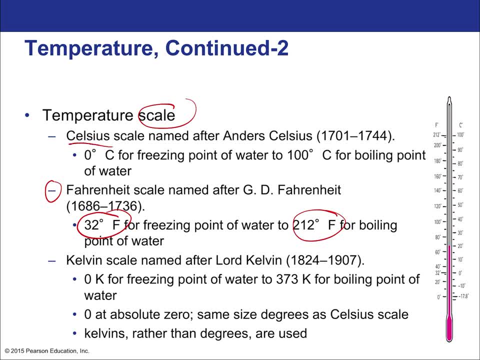 that's a pretty big. that's a pretty big jump, right, You know so. am I going to use a decimal? No, not in everyday language, but you can then describe those integer changes in the Fahrenheit scale. So definitely, it actually has its advantages as an everyday temperature scale. 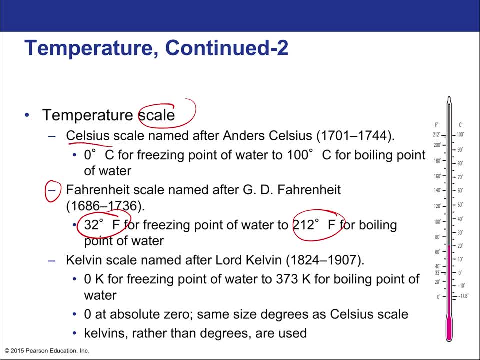 but it really is not well suited to chemistry or science. Okay, Now Celsius, we could say, is very well suited to chemistry. All right, Because it's got zero degrees Celsius for freezing and 100 degrees Celsius for boiling, All right. And I, and you know why do I, why do I say chemistry and 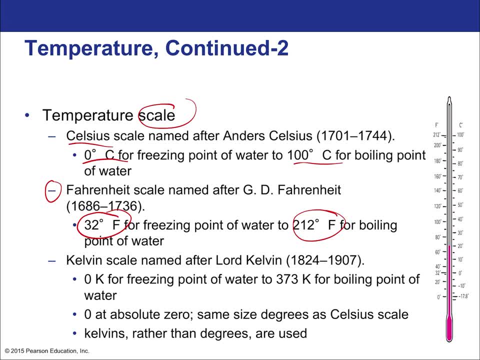 not physics? Well, because it is pretty much focused on taking experiments in a laboratory at sea level, because water only boils at a hundred degrees Celsius at sea level. right, And it's very much. that's not. that's not true in space. That's not a general statement, you know. so it is this. 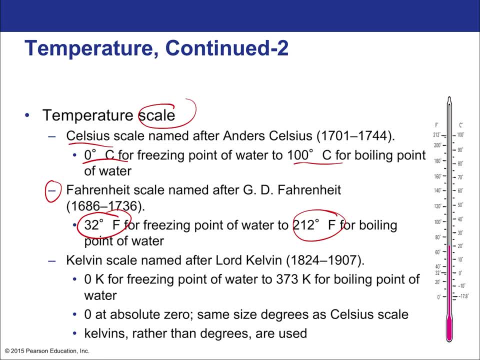 it's, it's focused on the properties of water, which are very important, you know, for in certain types of laboratory experiments. you know, certainly, and it has, it has advantages for that And it is widely used as the everyday temperature in most countries other than the United. 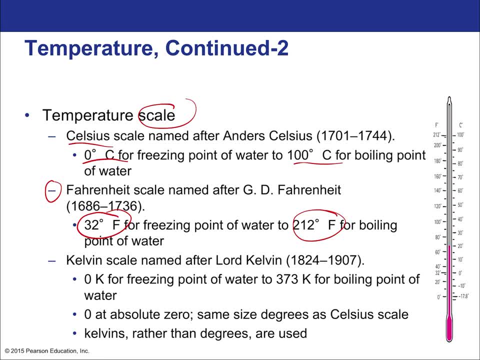 States, You know. so it has has been kind of adopted as a non-scientific type of temperature scale, but it still is a useful one, right? But it's very much focused on water, right, Water is incredibly important. But, you know, let's, you know, take, take that in consideration. Now the 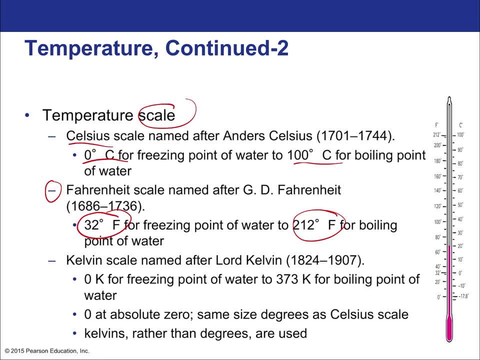 best temperature scale by far and one that is used by many of chem- by really most chemists, really, you know- but but certainly used by all physicists, is the Kelvin scale. All right, The Kelvin scale is really the scale we're going to talk about. It's the one we care about, All right. 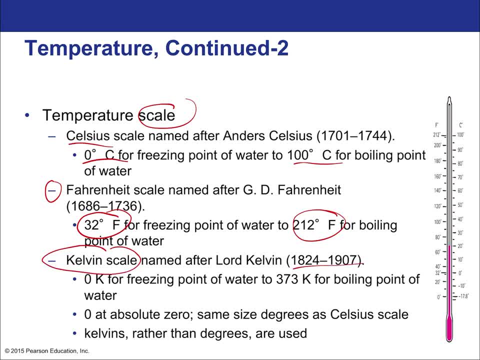 It came last. All right, Lord Kelvin, who lived from 1824 to 1907.. And what sets sets the Kelvin scale apart from the others right away is that zero degrees Kelvin is absolute zero. It is a theoretical value that can never be reached as far as we know, but represents the point at which 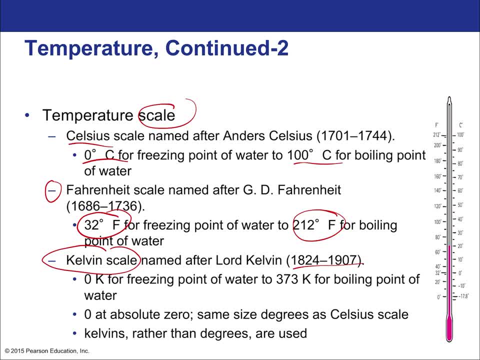 all molecular motion ceases. Okay, The change is the same as Celsius. So it did it kind of. it adopted something that was already used by the scientific community: the Celsius scale. so if you go up one Kelvin, that's the same as going up one degree Celsius. All right, And 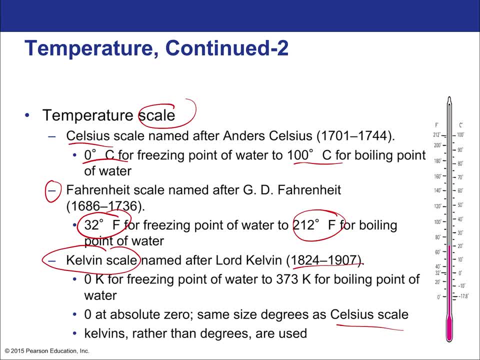 Kelvins rather than degrees are um, are used Okay, All right, Okay And um. what I mean by that is that when we talk about changes in Kelvin, we don't say degrees Kelvin, we just say Kelvin. 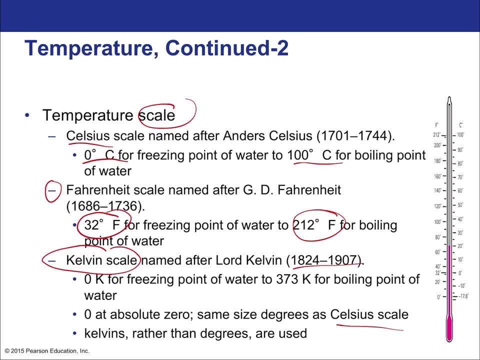 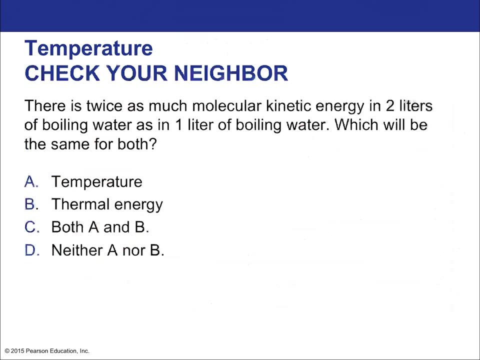 Okay, All right. So, um, by the way, um, boiling water is at um 373,, which means that freezing zero degrees Celsius is corresponds to 273.. Kelvin, Right, And that's a good kind of conversion factor there. Okay, So there's twice as much. 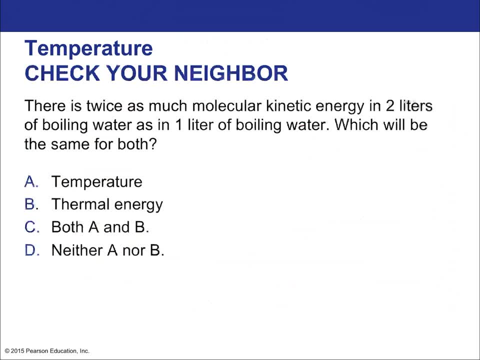 molecular kinetic energy in two liters of boiling water as in one liter of boiling water, which will be the same for both. Okay, Think about to have the definition of temperature. It's proportional to the average kinetic energy, So is it going to go up when there's more of a substance? What does 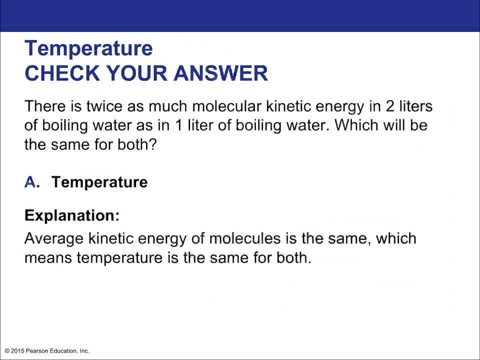 your everyday experience tell you: Definitely not. Okay, Temperature is independent of the amount of substance. Okay, It's proportional to a per particle quantity, Right? So that's, that's what we see. It doesn't matter how much you have with. 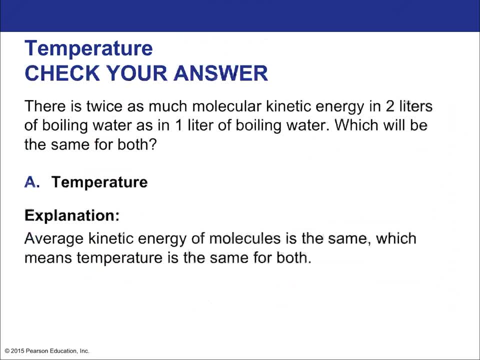 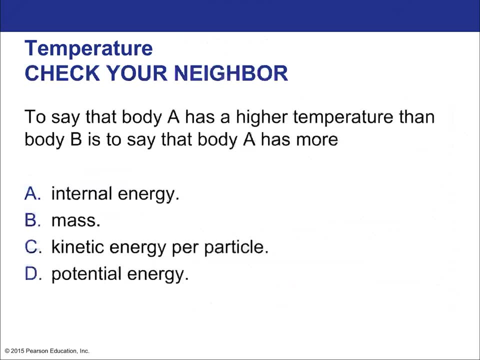 something. It just depends what the average part of that something is doing, whether it's that jiggling solid or that bouncing around gas molecule. Okay, So to say that body A has a higher temperature than body B is to say that body A has what Right? Well, I think you know. 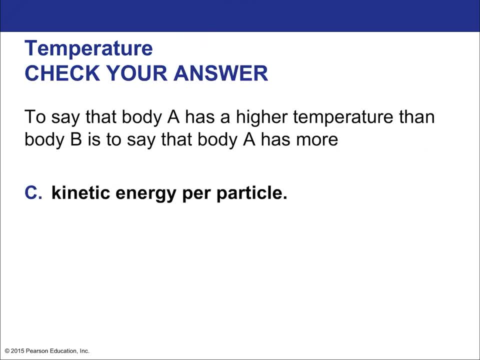 it right? If you don't, then you're not paying attention. It's kinetic energy per particle. Okay, That's a key idea, All right, And maybe you haven't thought about that being the really the definition of temperature, but it is. It's definitely one you want to take note of, Okay, So 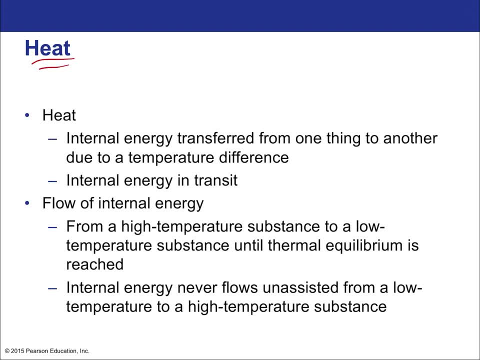 that's temperature, but let's talk about a different idea altogether, And that's heat. And heat is something we've already seen before, because heat, it turns out, is going to be measured in joules. Ah, so heat is an energy, All right. Temperature definitely is not The Kelvin. 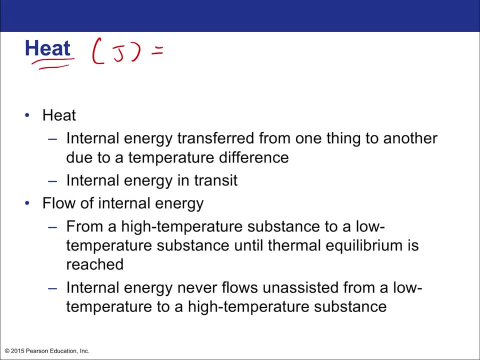 is a new unit at this point, Because if you think about the fact that the joule is just composed of units we've seen before, right, So that means we're going back to to mass distance and time, But that that joule, or rather that Kelvin, the Kelvin, is a new unit. 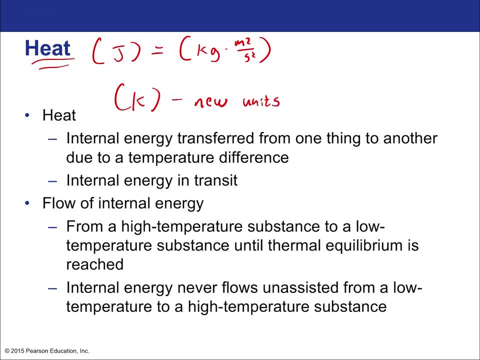 altogether. So if you're keeping count, that means at this point we have four units. Okay. We'll get one more before we really wrap up this semester, Okay, But you know that's because physics is all about breaking things down into the simplest ideas possible and saying that all you know. 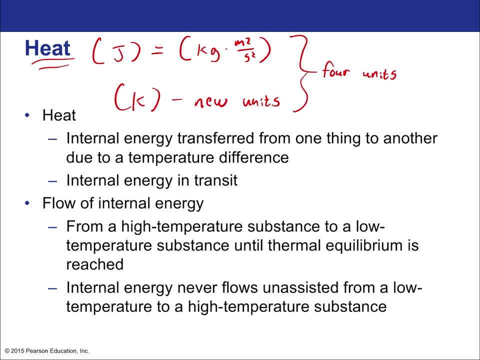 all the universe is described by basically five fundamental units is a pretty simple way of talking about things. right, It's a fundamental way. Physics is a fundamental science- Okay, All right, But anyway, heat is something we've talked about before. It's energy, And it's energy that has to do with temperature changes. Okay, Because 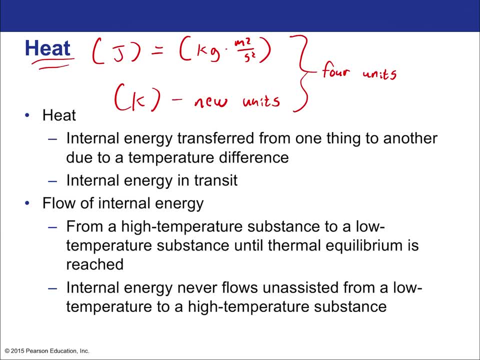 energy is all is just an accounting method, It's just a convenience, It's just a way for us, you know, to think about the world and make sense of it. It's not new physics in the way that Newton's laws are new physics. It's not new physics in the way that universal gravitation is new physics. 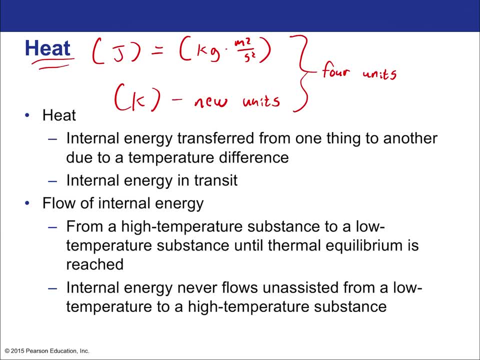 It's just convenient, Okay, And that's all energy is. And so then, if energy is going to be convenient, we should find a way to apply it to temperature as well, Okay, So hopefully you kind of see the motivation behind heat. nothing new, just a convenience, Okay. So what is it? It's internal. 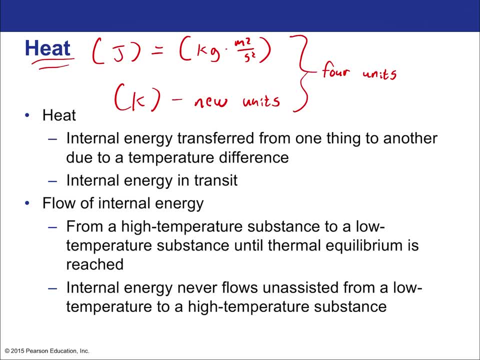 energy transferred from one thing to another due to a temperature difference, Okay, So energy, internal energy. So there's energy possessed by an object, Okay, Or a substance, or a system, whatever. whatever you know you may be looking at, you know you're looking at, you know you're. 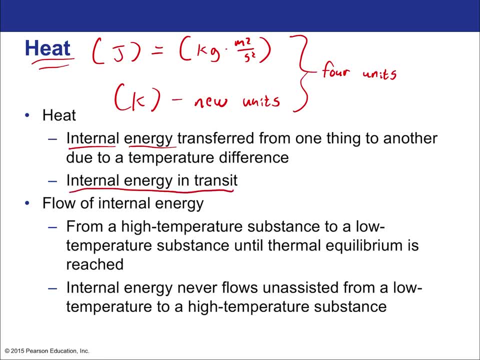 looking at: All right, And it's internal energy in transit. Okay, So it has to do with the flow, see transit flow. It's all about change. So from a high temperature substance to a low temperature substance, heat will flow. Okay, Until equilibrium is reached. So heat will flow from object A. 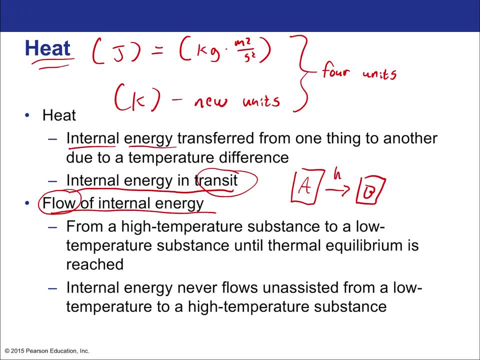 to object B, We'll have a flow of heat. All right, Okay. Internal energy never flows unassisted, unassisted from a low temperature to a high temperature substance. Okay, So there's a. there's always a directionality, We'll learn. 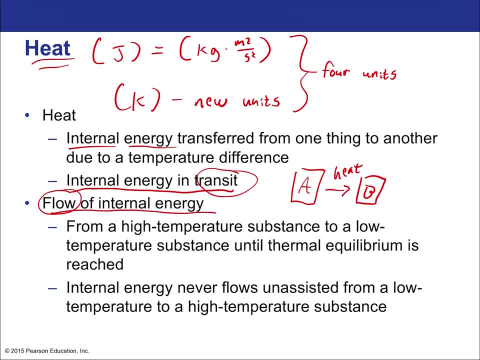 that that's actually part and parcel of the second law of thermodynamics. But for now we'll just kind of, you know, take, take that as gospel, Heat only flows in one direction. It flows in the downhill temperature direction. Okay, So internal energy would be possessed by: 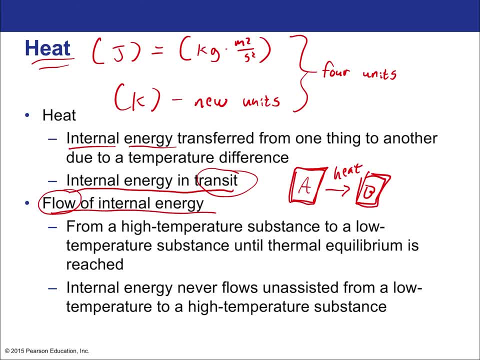 object A possessed by object B. heat flows between them. There's an analogy here, And the analogy is potential energy and work. Okay, So a force does work on an object, but an object never possesses work. An object possesses kinetic energy or potential energy. right, Potential energy being the best analogy to 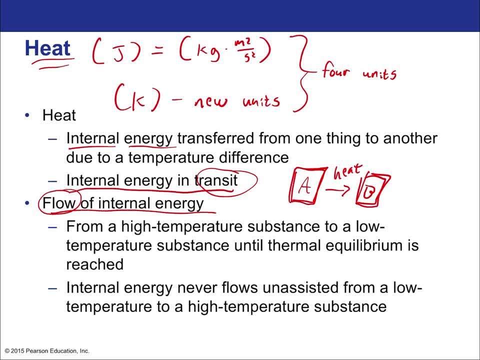 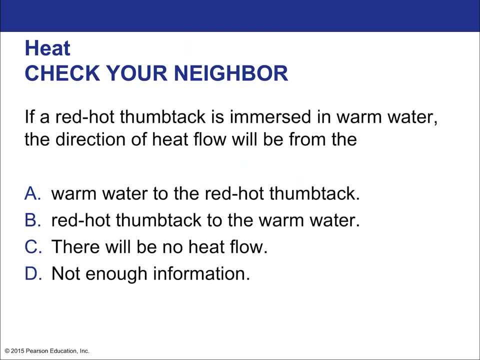 an internal energy because it has the potential to do something. Internal energy has potential to allow heat flow. So heat is like work. Internal energy is like potential energy. Okay, Makes sense. Okay, So in a red hot thumbtack, or if a red hot thumbtack is immersed in warm water. 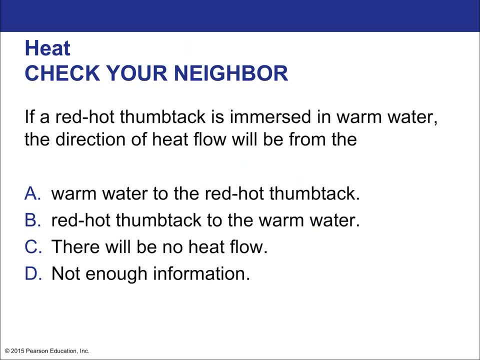 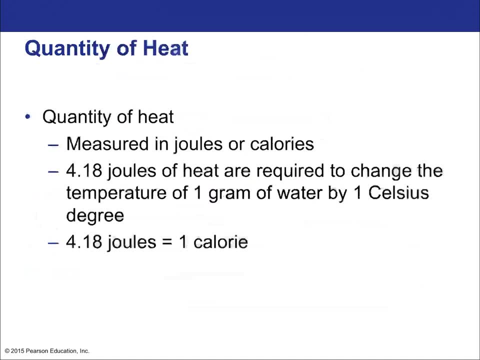 the direction of heat flow will be from. okay, think about the way it has to go. It's going to be from the hot thing to the cooler thing, from the red hot thumbtack to the warm water. All right, So let's quantify it some more. How do we talk about heat? Well, we can certainly measure in. 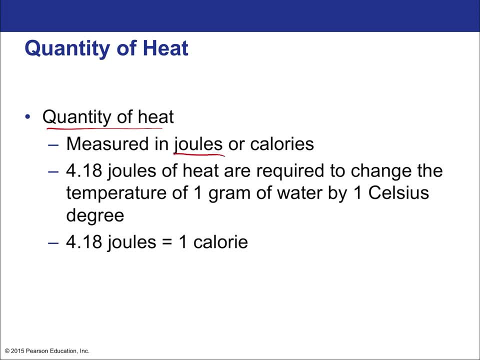 joules, right, We could fall back that, fall back on that as the sort of the basic derived unit because of you know, because again it is, it is a kilogram meter squared per second squared, but that is still, you know, very much a basic unit. 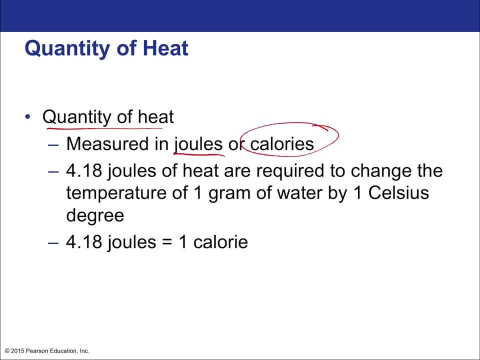 A calorie is another unit of temperature, but it is a it's it's not. it just has some conversion factor to a joule. All right, So this would not be composed of SI units. Okay, Think about: the calorie gets used quite a bit and you're going to be accountable for converting back and forth. 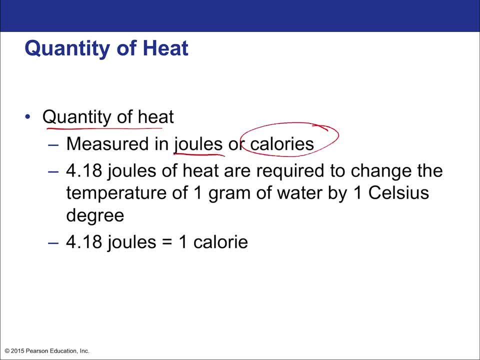 But Hey, as far as problems go, conversion problems aren't that bad right. So 4.18 joules of heat are required to change the temperature of one gram of water by one Celsius degree. That's how the calorie is converted to a joule. So 4.18 joules of heat are required to change the 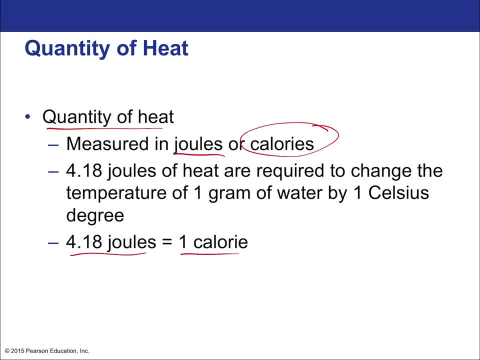 calories defined So that 4.18 joule is defined as the calorie, All right. Likewise, 4,186 joules is defined as the kilocalorie, All right. And that, by the way, is equal to the calorie with a capital. 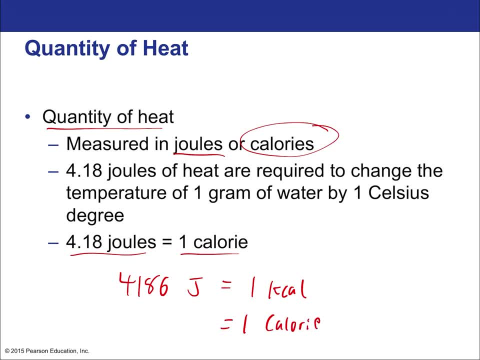 C and that's what you see on food packaging. So if you're eating a snack that has a hundred calories, that would be calorie with a capital capital C, which the rest of the world calls kilocalories, By the way, if you look at food packaging basically anywhere else in the world, 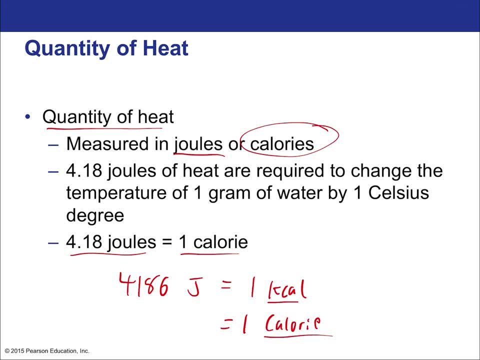 they don't call it calories, They call it Kcal, And that then would be equal to a hundred times 4,186 joules, or 400,000 approximately joules. That's too big right? Well, no, that's actually. 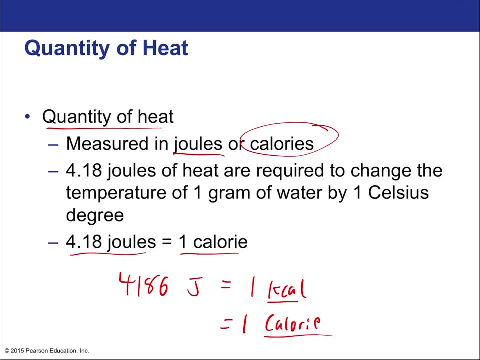 how much energy is in that food. It just goes to show that metabolic energy is huge, because 400,000 joules, I mean, that'd be like dropping a 4,000 kilogram car. Well, you know times, times a. 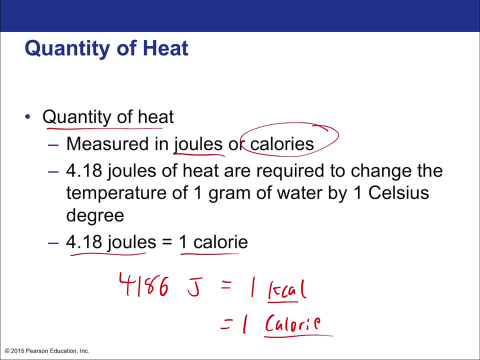 hundred meters. right, That's dropping a four. well, no, you have to multiply by 10. So 10 meters. So you take a 4,000 kilogram car. its weight would be 40,000 newtons, because approximately 4,000 times 10.. Okay, So again. 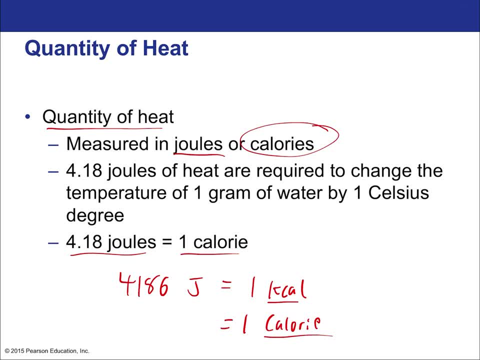 4,000 kilograms becomes 40,000 newtons on the surface of earth. And then work is, you know, is weight, times, time in this way, times distance, excuse me in this instance. So then multiply by 10 again, you got 400,000.. Okay, So again 100, too many numbers. Keep track about me, about me. 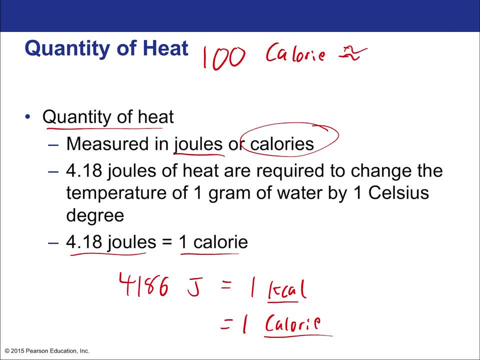 right now, 100 speculations, right? So 100 calories is equal to approximately 400,000 Joules. Okay, Well then, that would be equal to a 4,000 kilogramne car or large object— that's. 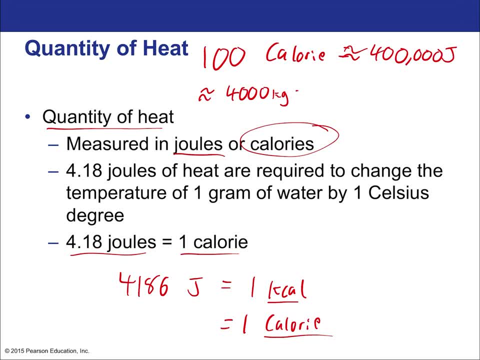 that's a huge object. 4,000 kilograms- right, That's like a big truck— times gravitational accelerations, which we approximate as 10 meters per second squared. and then times 10 meters. right, Because 4,000 times 10 times 10 is 400,000.. Okay, because it's just 4,000 times. 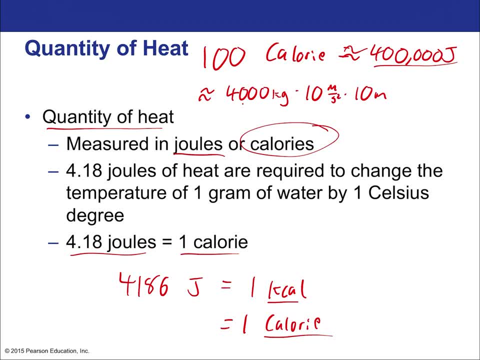 100.. All right, And so that would give you the- you know the correct units of dropping this big giant truck 10 meters, and 10 meters like 30 feet, I mean, you think about that, you drop a big giant. 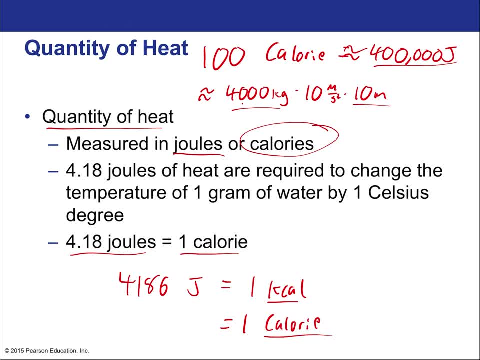 truck from 30 feet when it, when it hits the ground, I mean that's like a it's that's gonna make a huge giant dent. I mean there's gonna be a huge release of energy. you're gonna hear a giant smashing sound. I mean, think about how much energy that is, That's how much energy there's. 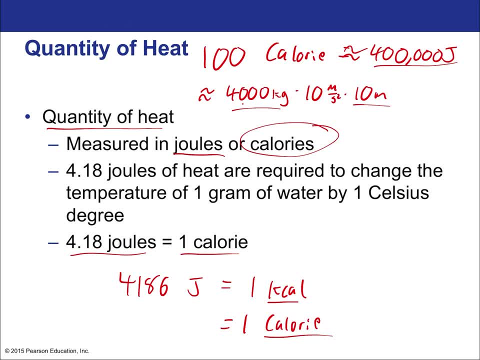 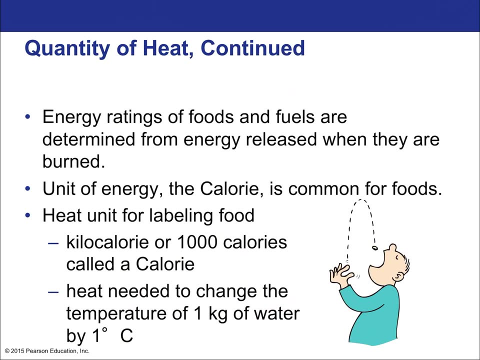 in 100 calorie snack. That's amazing, That is mind boggling. Just what's happening at the chemical level in a metabolic machine, like, like you know, like a mammal. It just it's so much energy. Okay, All right, All right. I mean, biology is amazing, amazing like that. Okay, so anyway. quantity of 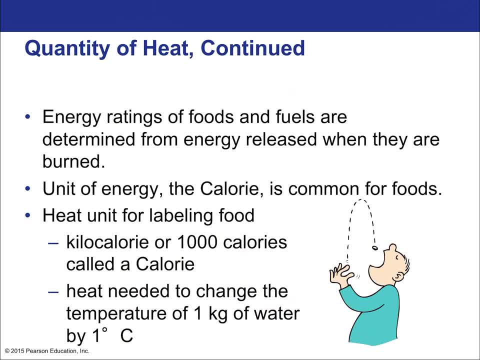 heat. continued. Energy ratings of food and fuels are determined from the energy release when they are burned. Okay, that's what I'm getting at, about eating a food, right? So the unit of energy, the calorie there it is in capital C- is common for foods. So the heat unit for labeling foods, the kilocalorie. 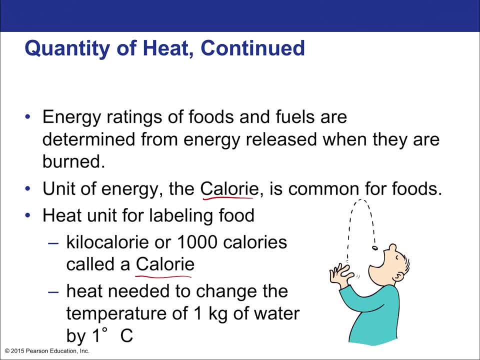 or 1000 calories is called a calorie right. That's what exactly what I was talking about. Heat needed to change the temperature of one kilogram of water one degree Celsius. Okay, so, instead of one gram, because it's 1000 times as much. Okay, so the same quantity of heat is. 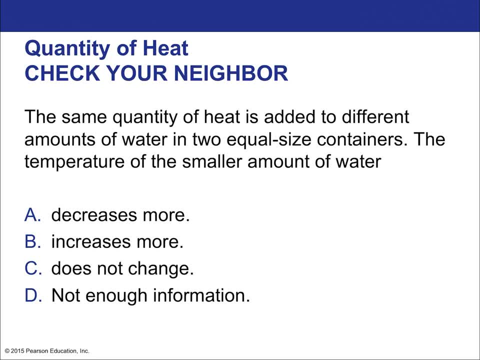 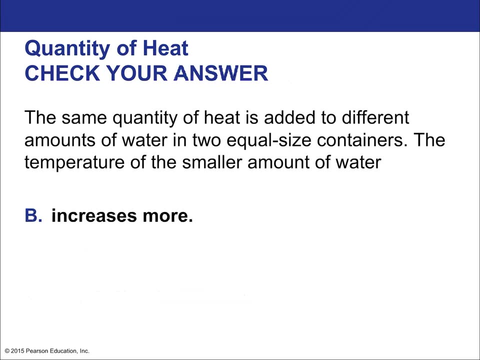 added to different amounts of water in two equal size containers. the temperature of the smaller amount of water, All right. Well, what happens? Does it decrease more? increase? more does not change, not information, What do you think? Okay, it increases more, All right, Because having less mass means less heat is needed. Okay, we saw that it was. 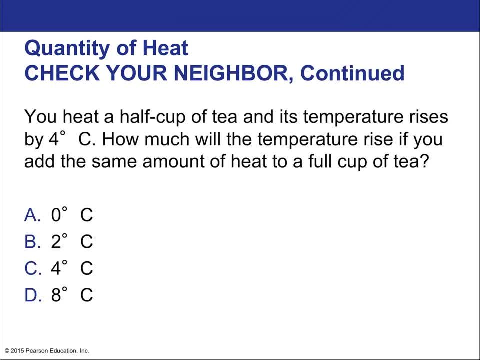 dependent on the amount of mass. right, That makes intuitive sense. Okay, so you heat half a half cup of tea and his temperature rises by four degrees Celsius. How much of the temperature rise if you have the same amount of heat to a full cup of tea? All right, but you have a guess. Absolutely, It's. 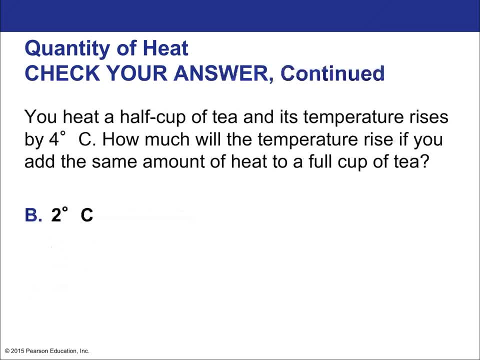 proportional Right. Double the mass would have to double the energy if you want the same temperature change. Okay, so you see, you know- and this is just based on that definition- the fact that the calorie is defined as you know, how much he eats, the heat it takes. So that's why, that's why I'm saying there's 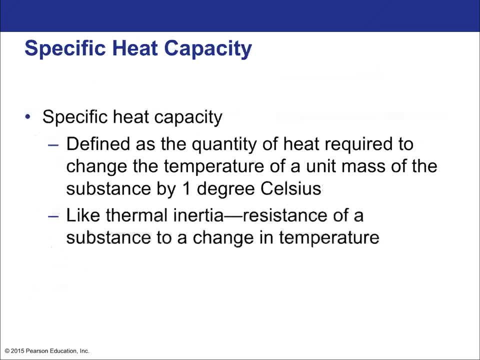 a direct portionality. Okay, All right. well, we can actually quantify that direct proportionality, And we can do it with the definition of specific heat capacity. This is just going to be a way to talk about how much energy it takes per degree per gram to heat something up, or per Kelvin per. 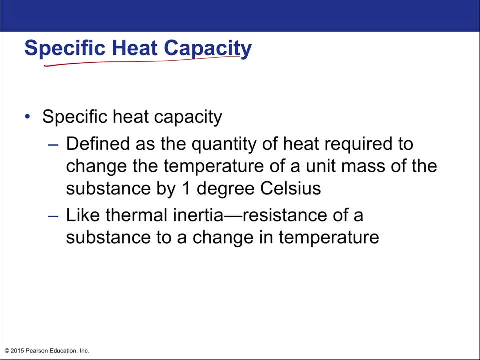 kilogram to heat something up. Okay, so specific heat capacity. what is it? Well, it is defined as the quantity of heat required to change the temperature of a unit mass of substance by one degree Celsius. And, by the way, a delta degrees Celsius is equal to a delta Kelvin. Okay, and 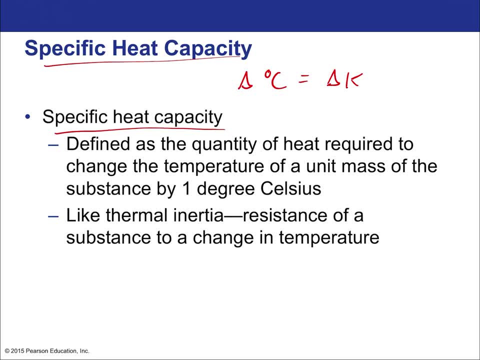 that's a great thing about changes, Because you know sure we have to remember that. you know zero degrees Celsius is 273 degrees Kelvin. you know you got to make sure you get that right in certain cases, But in many cases if you're only interested in a change of temperature. 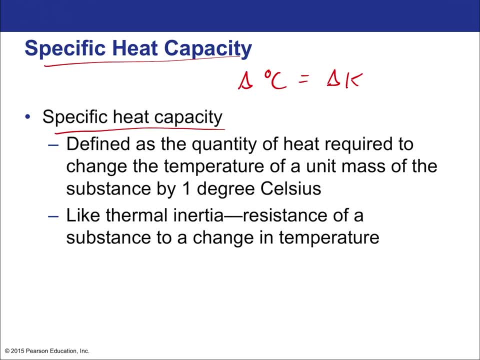 you don't even have to worry about converting from Celsius to Kelvin or from Kelvin to Celsius, because you're good to go, because the changes are equal, All right. Okay, like thermal inertia- resistance of a substance to change in temperature. Okay, so that's a great way to think about it. 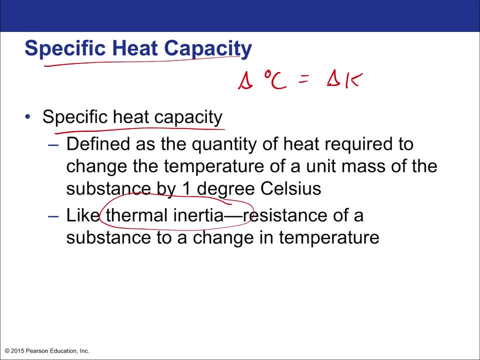 Let's unpack that a little bit: Thermal inertia. Remember inertia was the sluggishness of matter. the more massive something is, the harder it is to accelerate it. Same idea here: the more the more heat capacity a substance has, the harder it is to heat it up, the more energy it takes to heat it up. 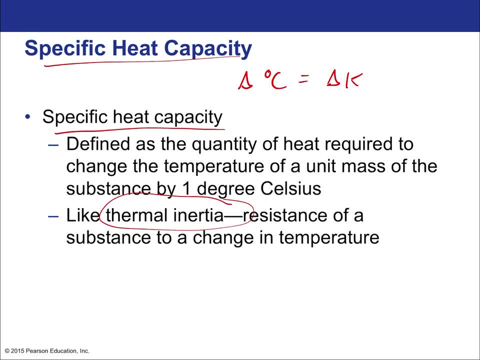 one degree or one Kelvin. So that means that as we look at different substances, we should expect some substances to have higher heat capacities and others All right. So think about something that's really easy to heat up. You're thinking of something, something that gets heat, that gets hot. 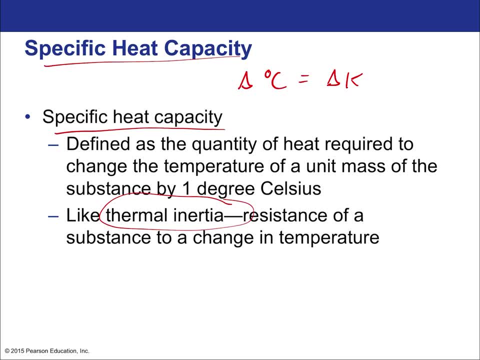 really easily. Okay. metal, right. Certain metals. you leave them on the sun, they're hot to the touch. really easily, Right. So that means that a metal must have a low specific heat capacity. it must is not literally its mass, it's just the quantity of that particular substance. Okay, Now what about? 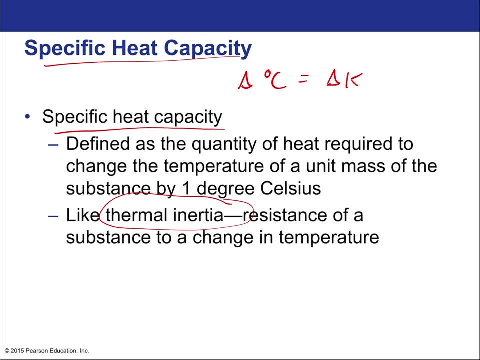 something that has really high thermal inertia, that has a high specific heat capacity, something that doesn't heat up very easily in the sun. Well water, right, You know, water is still cool to the touch even when it's been out in the sun, Right, Okay, All right. So different substances have 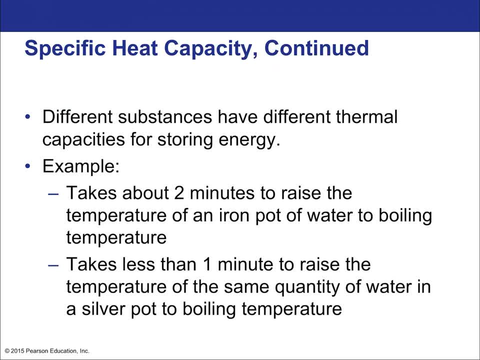 different thermal capacities for storing energy. Example: it takes about two minutes to raise the temperature of temperature of an iron pot of water to boiling temperature. and the minutes here don't. don't think here that we're saying that that heat capacity is fundamentally a time dependent phenomenon. We're just assuming that this is two minutes of adding. 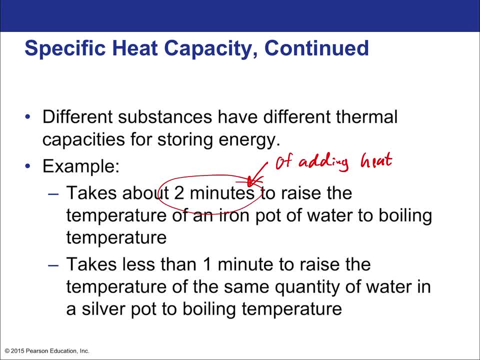 heat at a fixed rate. Alright, so that the time here is just kind of a convenience, a way to visualize something, to actually think about it in real terms. But there's not an actual because it depends on the rate. So we need to assume that we're adding heat at a steady rate, Okay? 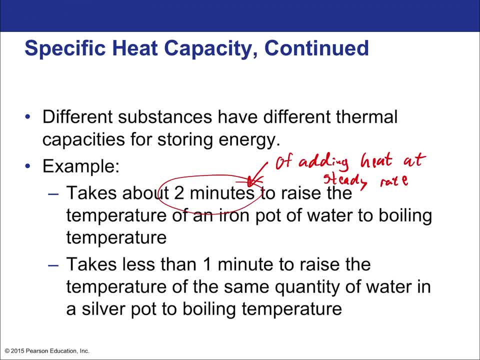 And we'd send add heat at that same steady rate to to water in order to make this comparison right. So it takes less than a minute to raise the temperature of the same quantity of water in a silver pot to boiling temperature. Okay, So continuum of heat capacity right. getting to the 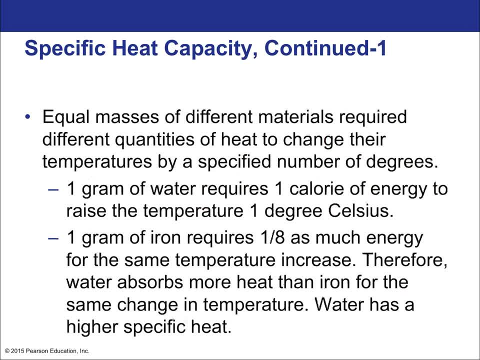 actual, quantified the equation, the way we're going to actually solve problems. equal masses of different materials require different quantities of heat to change the temperatures by a specific number of degrees. Okay, I'm basically said this, but it's good to put it: have it in a confined. 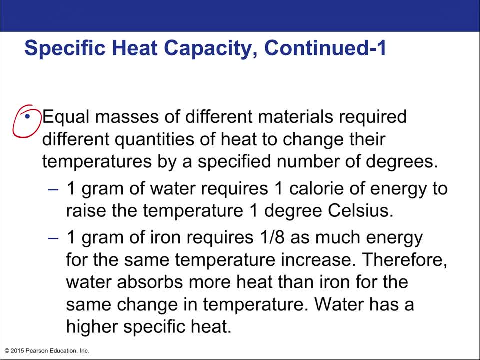 sentence like this: Okay, It defines and confines sentence. One gram of water requires one calorie of energy to raise the temperature one degrees Celsius. okay, we've established that right, And that is 4.186 joules, All right. so one calorie is 4.186, 86 joules, All right. 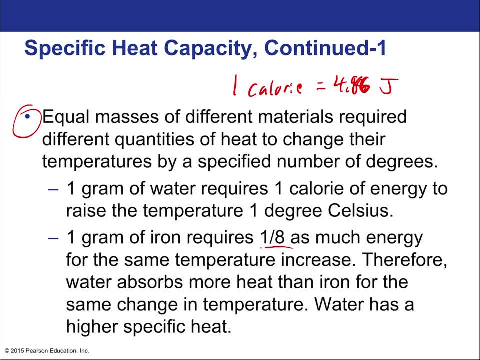 one gram of iron, on the other hand, what cards one eighth as much? there we have a direct quantified comparison between the two. as much energy for the same temperature increase. therefore, water absorbs more heat than iron. for the same change in temperature, water has a higher specific heat. 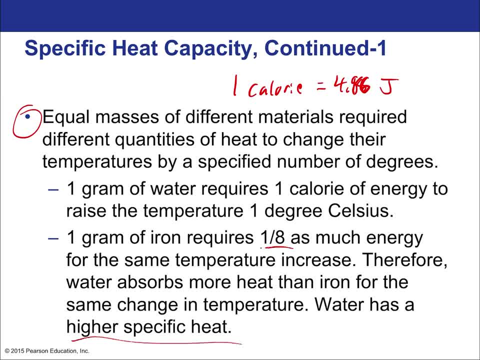 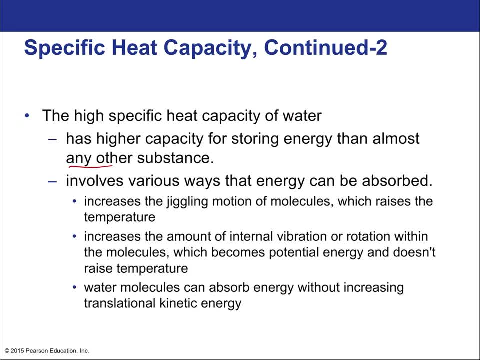 okay, so how much? you know it would take one-eighth as much energy. okay, so the high specific heat capacity of water. it has a higher capacity of restoring energy to almost any other substance. really, it's remarkable. all right, and the only other really even remotely common substance. 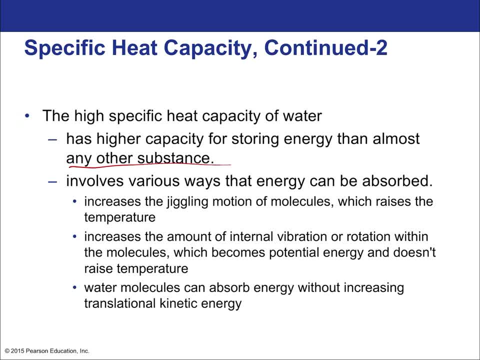 that has a higher heat capacity and really i mean you can. you can look at all kinds of of different chemical combinations, but the one out there is liquid ammonia. all right, liquid ammonia like you would find on um titan, the moon, the one of the moons of saturn, the only moon in. 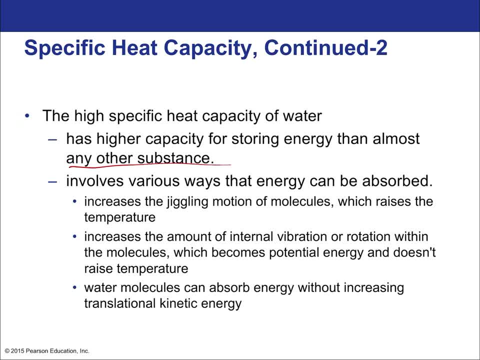 our solar system that has an atmosphere, interestingly, but that that moon has lakes of liquid ammonia and that those lakes have a higher heat capacity than water. all right, um, that's that's about it. true, truly and honestly, there's no metals that have higher heat capacity. 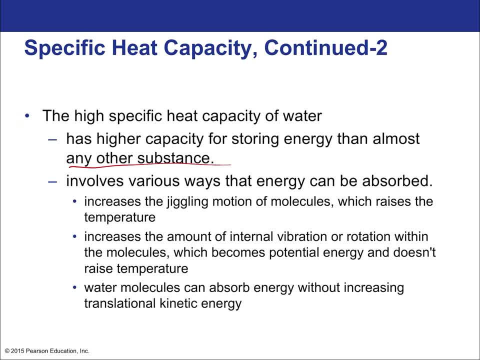 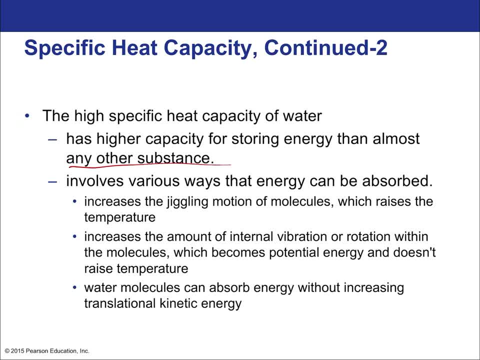 absorbed. so essentially, the molecules have lots of ways they can absorb the energy. they can- uh, they can, um, increase their jiggling motion, um, they can increase the amount of inertial vibration. a water molecule can absorb energy without increasing translational kinetic energy. so because of that complicated way that all the molecules can interact and absorb that energy, 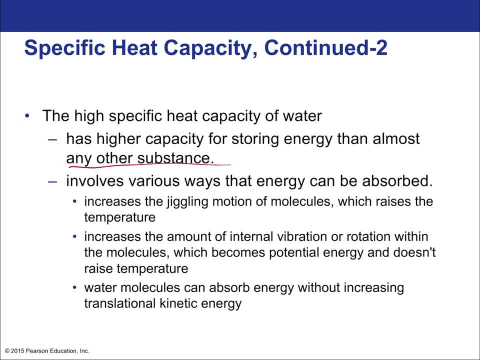 that means that they're not translating and bouncing around much, they're doing other things, that energy is going to other places. so, at the molecular level, at the level of treating molecules like, like little combinations of masses and springs, okay, that that. that's the explanation of why water has such a high heat capacity, which is a neat way of thinking about it. okay, it's not. 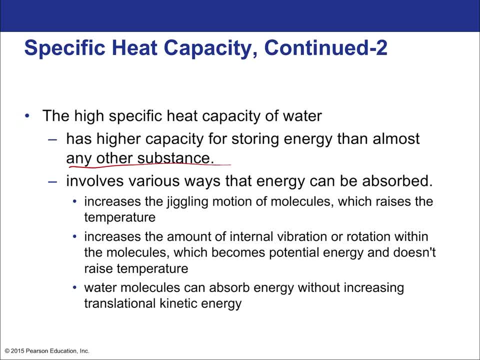 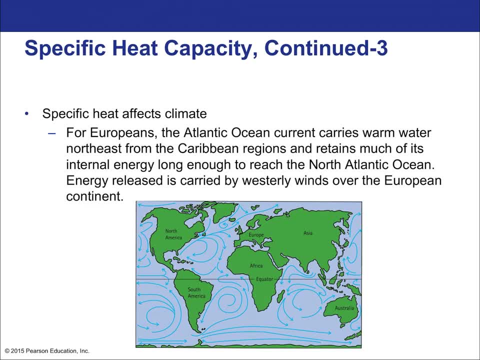 the primary way we think about heat capacity. we're mostly just going to worry about the macroscopic consequence of it, but if you're curious about why water has such a heat capacity, this is the kind of quick summary. okay, so specific heat capacities affect climate. all right, so this is the idea that the, the oceans have being 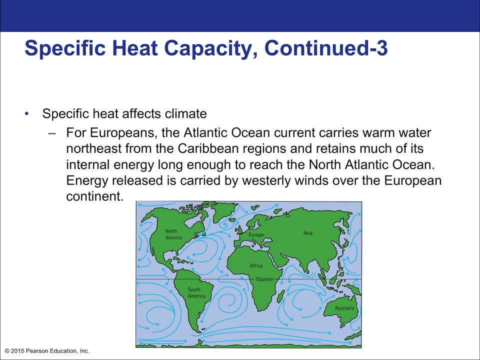 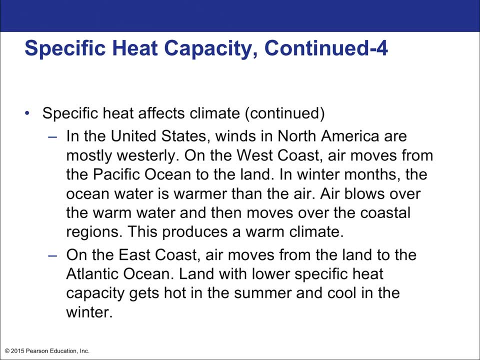 such a sink for heat capacity being able to absorb so much energy, they can drive big climate effects. that's where you get things like the jet stream. all right, um, i'm just gonna let you read over this example. it's fascinating, but we, you know, i'm gonna focus on the main, the main topics here. 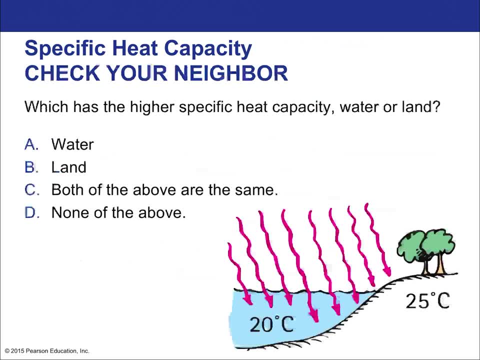 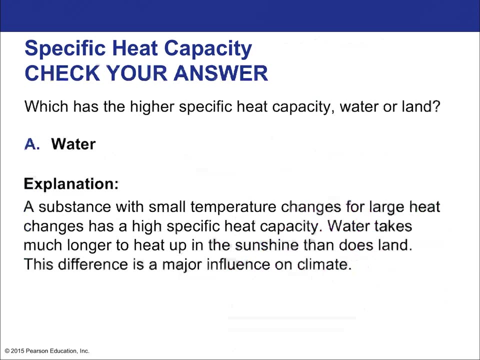 okay, and but here's a good example that i do want to make sure we can, we can cover. so which has the higher um specific heat capacity? water or land? you know the answer: water, of course. okay, absolutely right. so you know, between a lake and the shore, the water has a much higher heat capacity. it's going to be able to absorb a much. 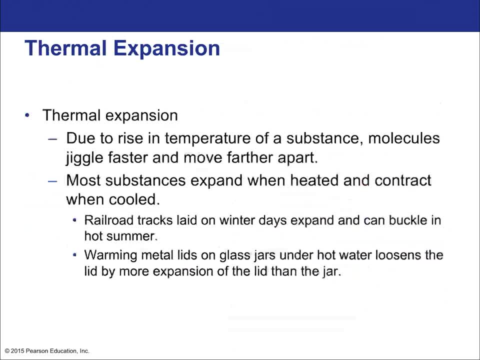 more energy for a temperature change. okay, all right. so on the thermal expansion. so, due to the rise in temperature of substance, molecules jigger, fat jiggle. they jiggle faster and move further apart. all right. so even solids, you know whether they're all kind of fixed in place? they're not. 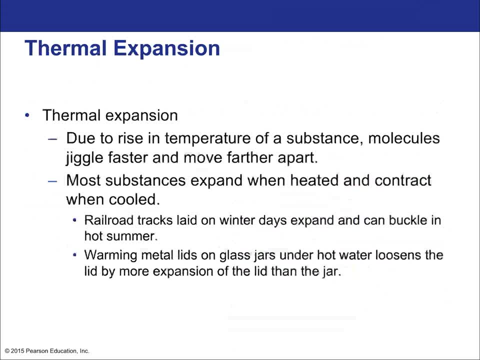 going to be able to absorb as much heat as they would if they were to absorb as much heat as they would. okay, so most substances expand when heated and contract when cooled. okay, there are some exceptions, but absolutely so. railroad tracks, for example, laid on winter days, expand and can buckle. 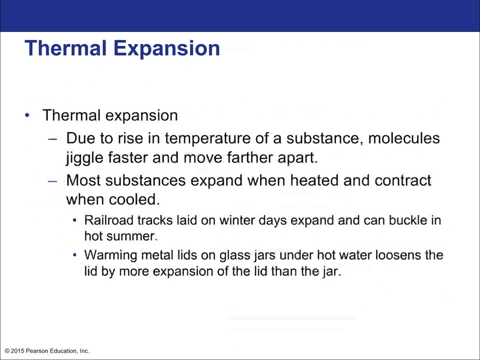 in the hot summer. that's why they're laid with gaps between them if you look at- look at- railroad tracks. okay, warming metal lids and glass jars under hot water loose loosens the lid by more expansion of the lid than the jar. all right, that's a good way to get get the um. 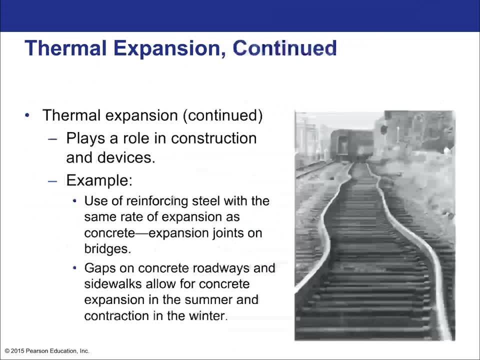 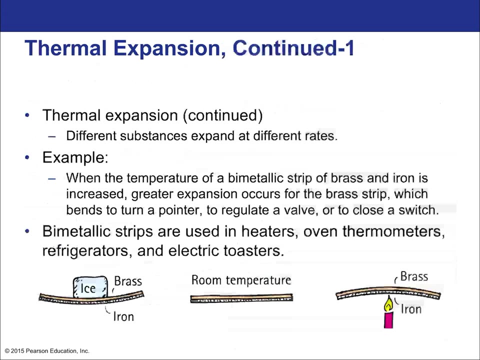 the lid loose, all right, so all right. here's an example of a railroad track that was not not enough. gaps were created, all right, and it absolutely buckled underneath the on a very hot day. okay, so thermal expansion can cause bending and can be a mechanism of a very basic type. 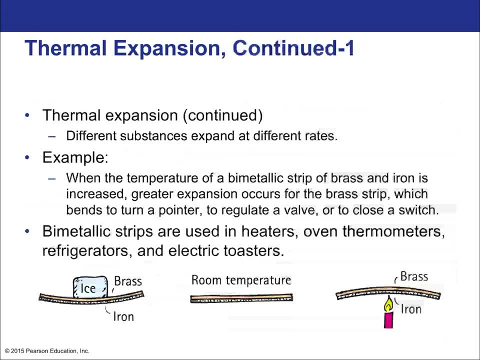 of thermometer, and so this is the idea of a bimetallic strip. okay, so different substances expand at different rates, just like different substances have different specific heat capacities. there's something called the coefficient of thermal expansion, which is material specific. so when the temperature of a bimetallic strip of brass and iron is 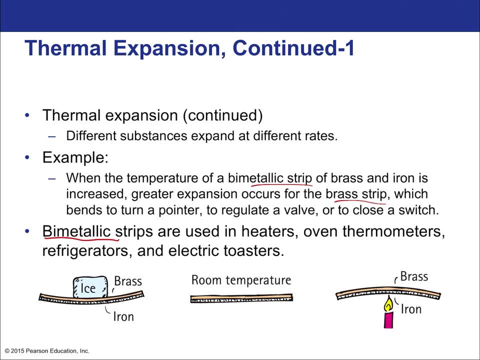 increased, the greater expansion occurs for the brass. so the brass has a ability to to expand more for the same temperature change, because there's going to be thermal equilibrium between the brass and the iron, but the brass stretches out more for that same temperature than the iron. all right, 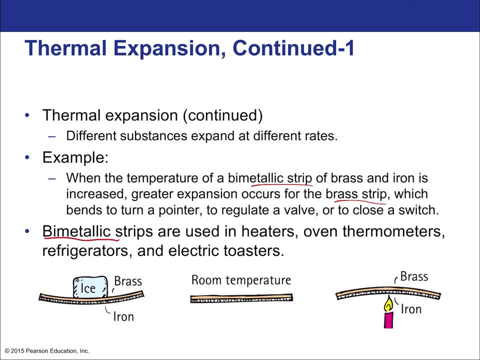 so that bends to turn a pointer to regulate a valve or to close a switch. all right, so it is a very effective temperature driven switch mechanism. all right. so here, for example, if we cool the whole bimetallic strip, then it's going to bend towards the ice. all right, because what's happening is the 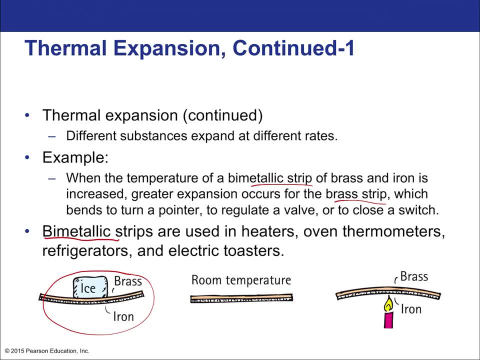 the brass is going to shrink more than the iron. that means that the curvature is going to be on the part that shrunk more. that's why it's curved this way. on the other hand, if you heat something up- and it doesn't matter which side you heat it up on- if you heat it up on the other side, it's going to. 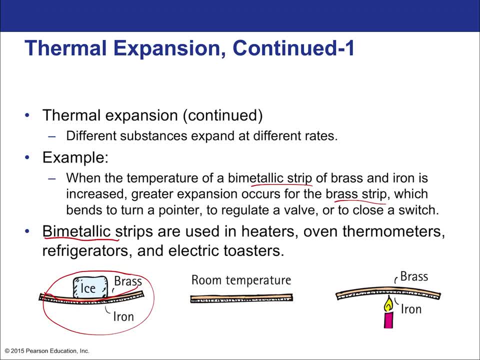 be on the inside of the curvature. but if you heat it up on the outside of the curvature, so that bad, then the brass is going to expand more, so then the brass is on the outside of the curvature. so cooling brass is on the inside of the curvature, heating brass on the outside of the curvature. 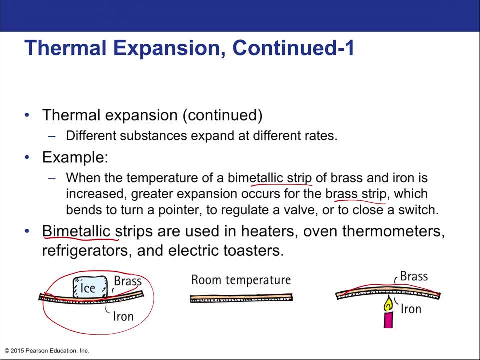 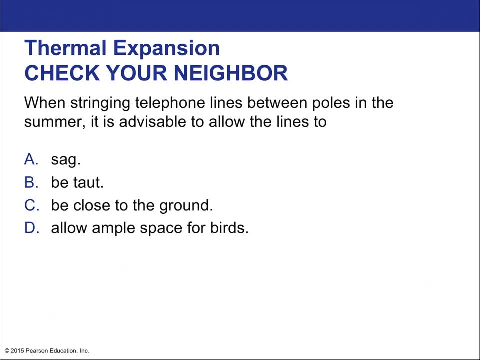 both explained by the fact that brass changes in length more for any temperature change, whether it's a decrease or an increase. okay, all right. so when a stringing telephone line between poles in um, or wind stringing telephone lines between poles in the summer, it is advisable to make sure that the 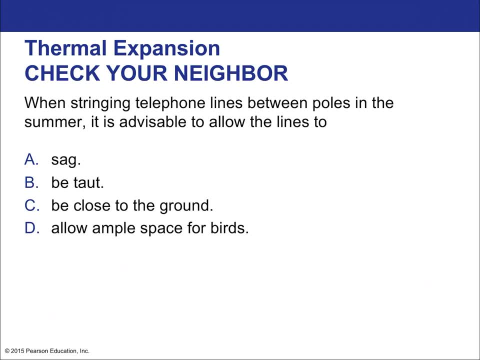 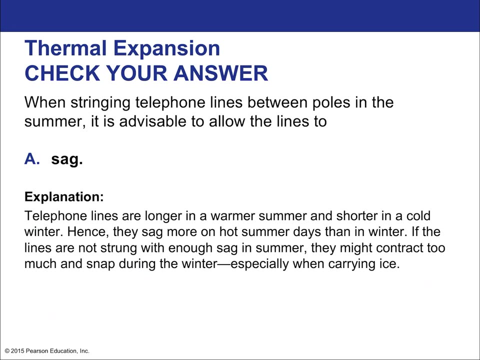 to allow the lines to do what. okay, so what's gonna happen? think about the summer. what's gonna be the state of the telephone lines compared to in the winter? okay, sag right, because they're they're expanded, they're longer than they will be. what's gonna happen in the winter? they're going to contract to a to. 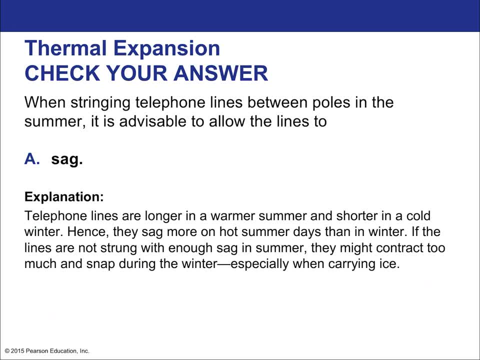 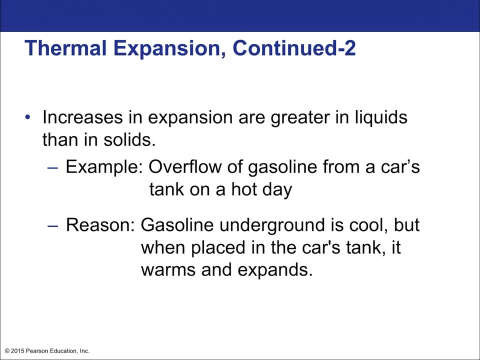 a length that's shorter if you had. if you attach them taught in the summer, they're gonna snap in the winter. okay, so thermal expansion is it. increases in expansion are greater in liquids and solids. all right, significantly. so all right, solids we're talking. you know less than. 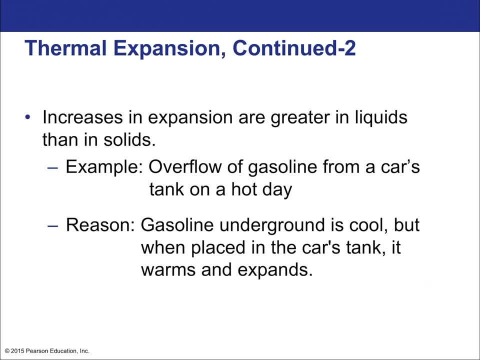 1% in terms of the actual- you know- change in length, for example. but liquids it can be much more dramatic, gases even more so. so overflow of gasoline from a car's tank on a hot day, okay, because we've got. if the the liquid gas, it's. 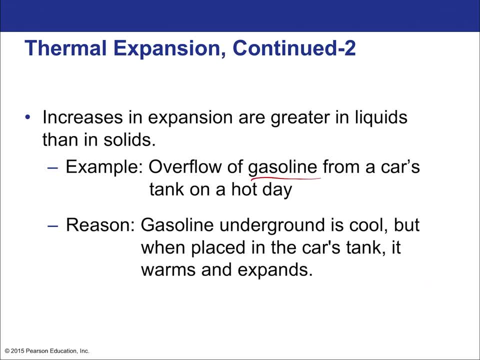 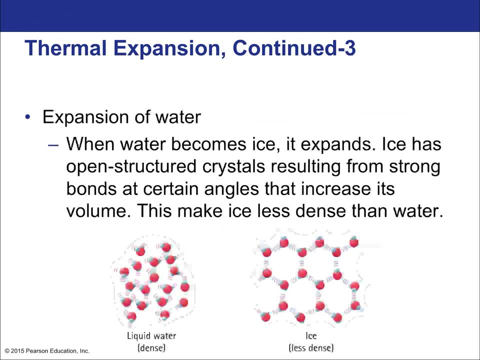 very hot, right, because we course gasoline, but of course it's a liquid, all right. gasoline underground is cool, but when placed in the car's tank it warms and expands, all right. here's an example of expansion of water, right, so water is an interesting case. so 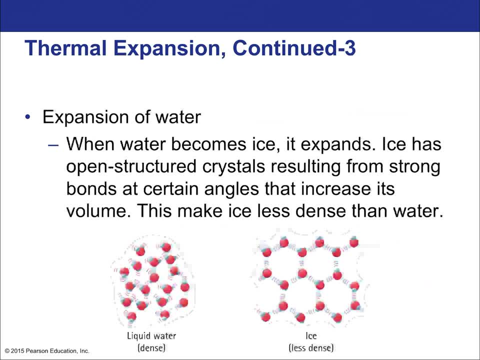 when water becomes ice it expands. ice has an open structured crystal which results from strong- we can't strong- bonds at certain angles that increase its volume. this makes ice less dense than water. that's unusual for solids. solids are almost always denser than the liquid. than their liquid state, water is. 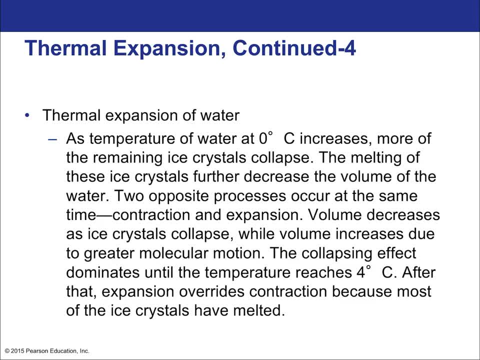 the exception, all right. furthermore, thermal expansion water has another oddity, besides ice being less dense than the liquid as temperature of water at zero degrees. so this would be water that's just melted, okay, but so at zero degrees you can have, and we talked about what we talked about. 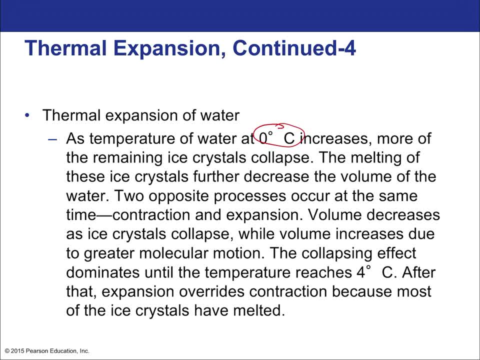 phase changes a bit more later, but we have zero degrees. you can have both a solid state and a liquid state for water, right again at atmospheric pressure, because you know, of course freezing is dependent on the pressure. but let's assume that we have, you know, liquid at zero degrees. so more, more of the 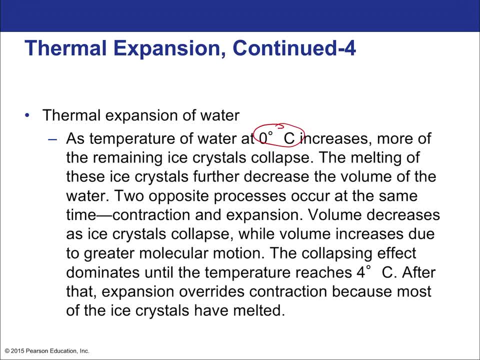 remaining ice crystals collapse, okay. the melting of these ice crystals further decreases the volume of the water. two opposite processes occur at the same time: the contract contraction and expansion. alright. so volume decreases as the ice crystals collapse, while volume increases due to the greater molecular motion. the collapsing effects: dom the collapsing. 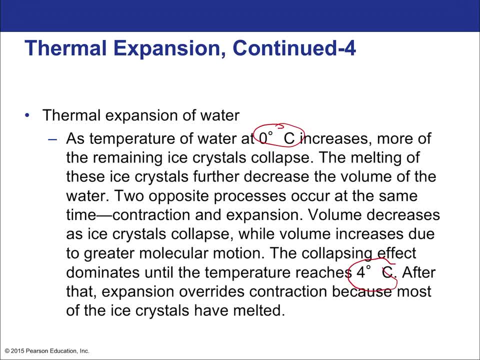 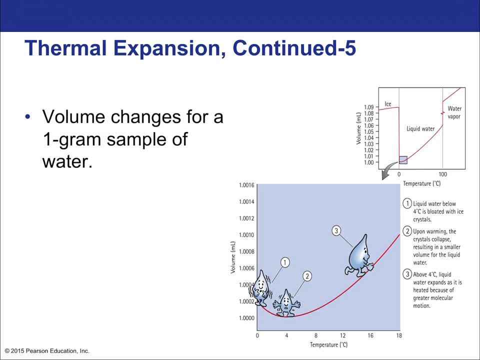 effect dominates until the temperature reaches four degrees Celsius. after that, the expansion overrides the contraction, because most the ice crystals have melted. what this looks like on temperature scale then is we can look, and if we zoom in, at the temperature difference between zero and eighteen degrees Celsius, alright, 18 is still pretty cool. alright, you know it's getting on the 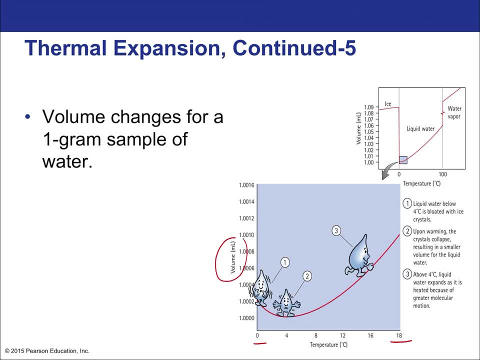 warm side we can see that there is a dip in the density that occurs between zero and four. so point two is the least dense that water can be alright. so four degree Celsius water is the least dense, alright as far as the liquid state. after that it's going then. it's then going to start. 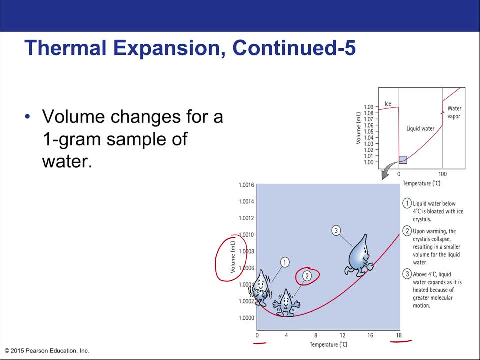 or, excuse me, I kept saying least dense. correct myself. there it is the most dense because after that the density in the disease then going to decrease, because the volume of IMC and the density will continue to decrease as the water becomes warmer, warmer now. is it a big dense? is the big density change will look at the volume. 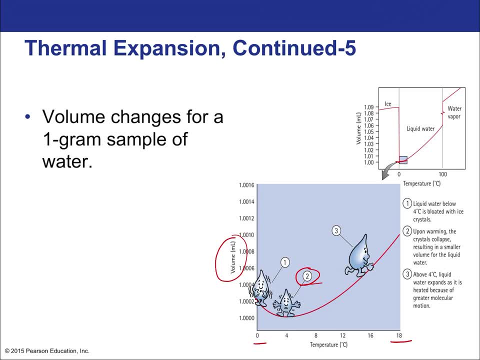 absolutely not right. so if we go from zero degrees up to right to the point where it starts to boil, we can see that there is a damper, there is a dense exchange of only about six percent. okay so, because a volume that did take up a space of one liter. 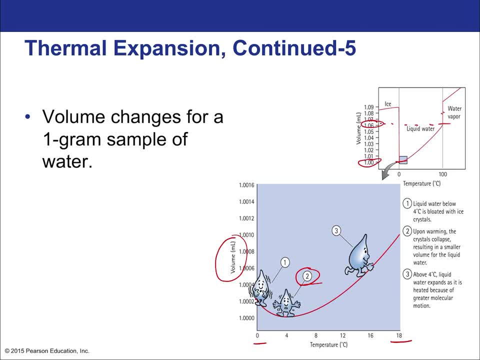 now takes up a space of 1.06 liters, but the mass hasn't changed, all right, so the volume has increased by six percent. the mass has not changed. therefore the density, the density change has been the reciprocal of 1.06, all right, so not not quite, as not quite a six percent reduction, but a you. 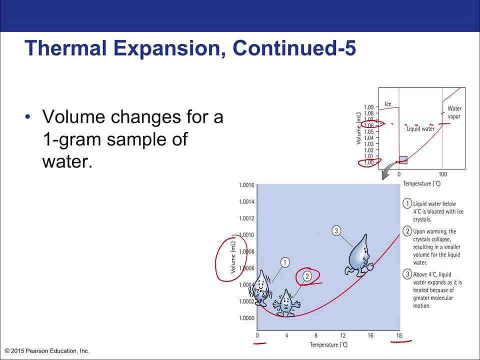 know less, definitely less than ten percent reduction in the density of the water. okay, so not not a big difference. and that's between water that went from zero degrees all up to being about ready to boil. so water is about ready to boil- is measurably less dense. okay, because it's taking up. 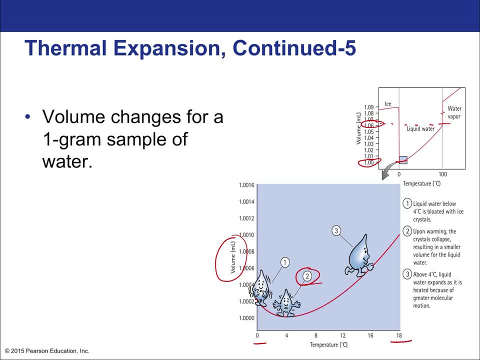 more space, not a lot, but you know something in the low percentage. low percentage is less than ten percent, and so that means that this difference between zero and four is smaller still. you can see it's point: zero, zero, two, right, so it's actually a very subtle effect. 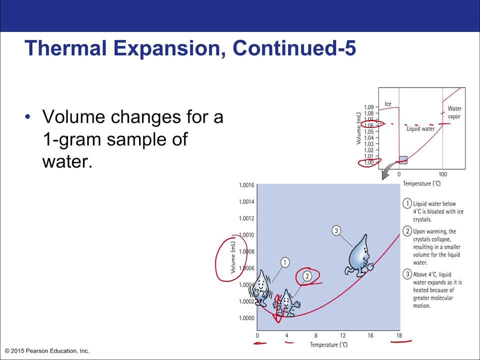 and it'll only matter for, you know, certain, certain cases. it kind of it's something we consider in the oceans and it's something you consider in certain experiments that you can get the most dense water at four degrees celsius. okay, but of course if you freeze water then the density 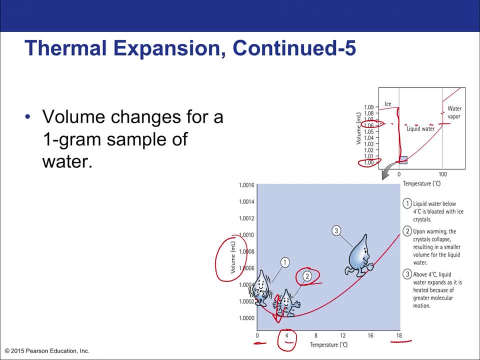 decreases quite a bit. right, it decreases up to almost ten percent because we have that ice is about, is about only ninety percent as dense as water. and then if you go another end, if you boil something, well then look it actually, the density, you know, becomes incredibly less because of course, gases aren't very dense, you know. it actually just defines. 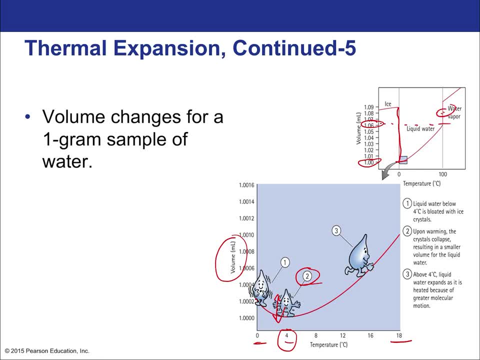 defined depends on how you can find them. and so then, of course, that's why we see there's a huge jump and water vapor, shown by the symbol here, that is no longer on the same scale. and then you know, water vapor is very, very low density, as it, you know, continues to just expand out to fill its 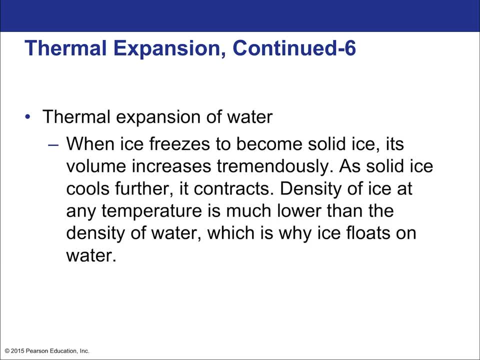 face. okay, all right. so thermal expansion of water. when ice freezes to become a solid, solid ice, its volume increases tremendously. As solid ice cools further, it contracts. Density of ice at any temperature is much lower, which is why ice floats. okay. So when a sample of zero-degree water is heated, 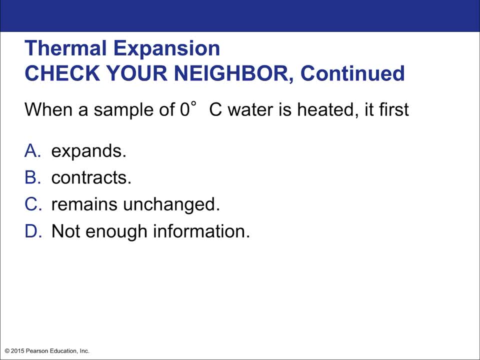 it first we talked about this. the density's gonna go up, which means it contracts okay, Until it reaches four degrees, and that's the densest water can be- all right, Liquid water When a sample of four-degree water is cooled. 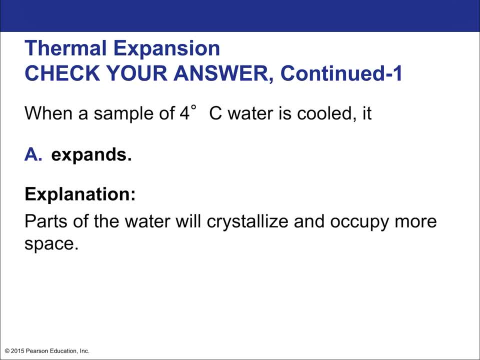 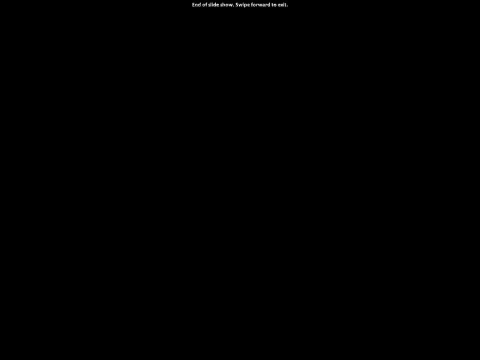 it. ah right, It expands. okay, It's actually gonna become slightly less dense, All right, so that's it We had. there's a brief introduction to a couple ideas. I have three ideas. What is temperature? How do we define it? 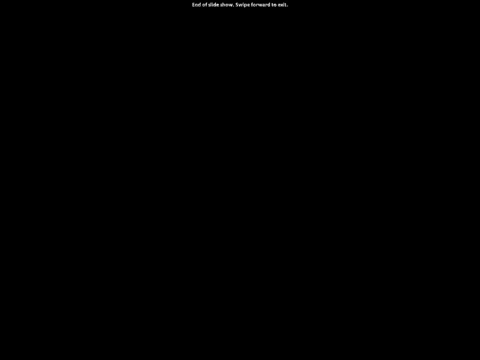 What is specific heat capacity And how it's really specific right? Different materials have different amounts of energy it takes to heat them up. And then, last of all, what's the idea behind thermal expansion? How does it apply to water as an important example of liquid?